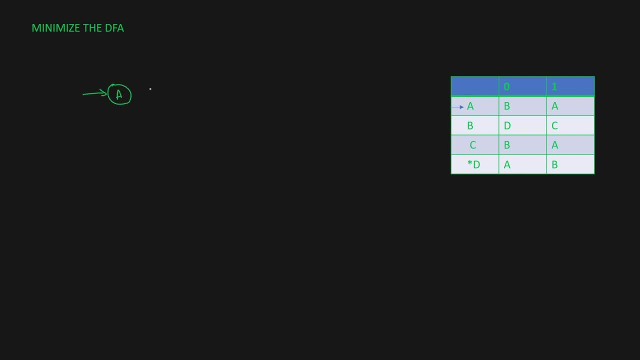 say: this is a starting state A And when we get input 0, you go to state B And you get input 1, you are staying in state A itself And in state B if you get input 0, you are. 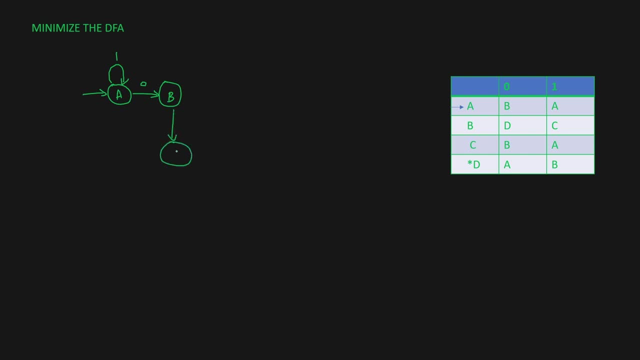 going to state D And since state D is our final state double circle, And you get input 1, you are going to state C. Now, in state C, if you get input 0, you are going to go to state B, So you get input 0, you are going to go to state C And you get input. 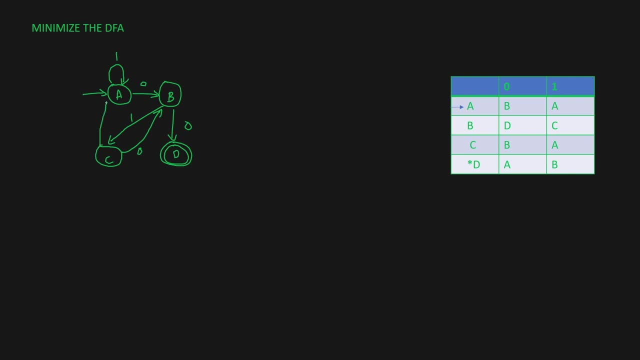 1, you are going to go to state A And in state D you get input 0, you go to state A And you get input 1, you go to state B. So this is our DFA. Now we have to minimize. 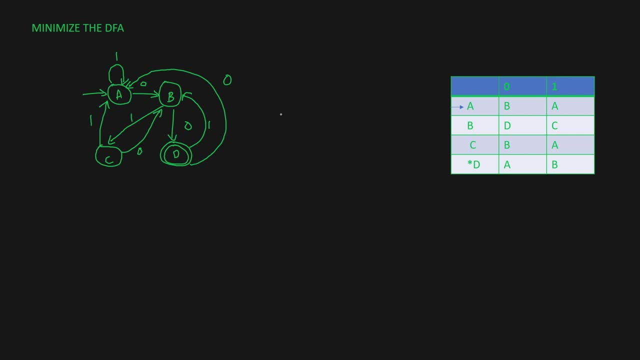 this DFA And we can see how many states we have. At least we can minimize it. Now we have to check for the equivalence of the states. So what we'll do is first we'll check zero equivalence. Now, what is zero equivalence? 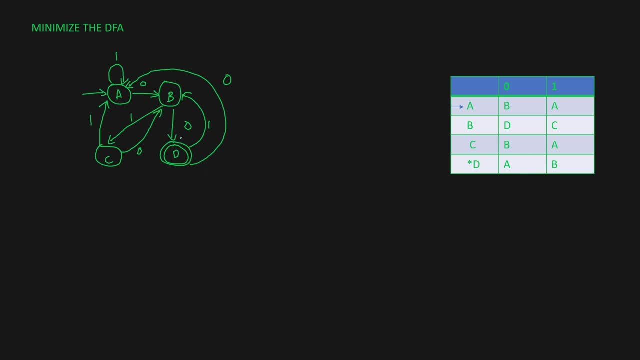 We have to check or divide the states in two groups, where one group is of all the states which are non-final states and one group is of all the states that are final states. So zero equivalence is like this: We have got A DFA. 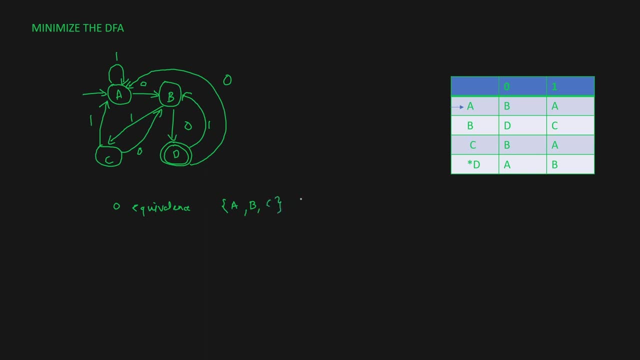 B and C, which are non-final states, And we have got D, which is a final state. So this is zero equivalence. Now, one equivalence is states when, depending on the input, we have to check: is the output part of the same set of states or not? 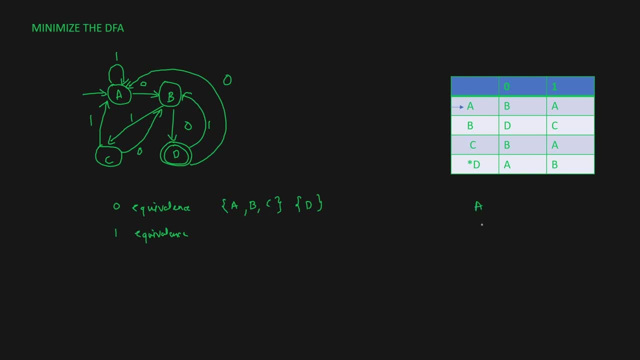 Okay, so let's say we have to compare A and B. So A and B. Now getting input zero in state A, we go to state B, Correct. And on input getting zero, we go to state B, Correct. And on input getting zero from B, we go to state D. Now are B and D part of the same set? 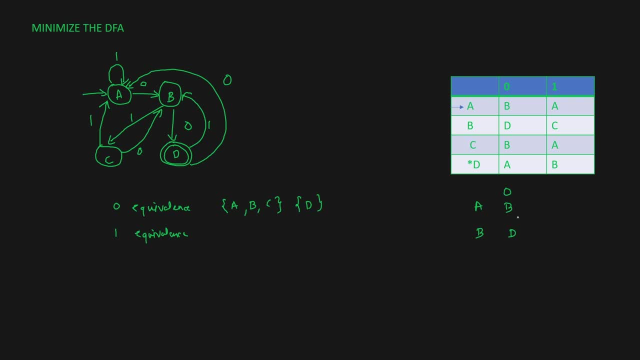 over here. No, B is in this set, D is in this set, So that's why A and B are not one equivalent. Okay, So A and B are not one equivalent. Alright, so what we'll do? we'll create a separate group over here for A and a separate. 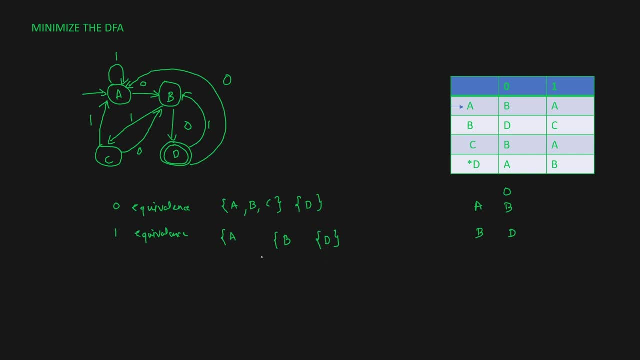 group over here for B And D is already present in the separate group. Okay, Now we have to compare A and C. Okay, So let's say A and C. On getting input zero, we go to state B, Correct, Okay. 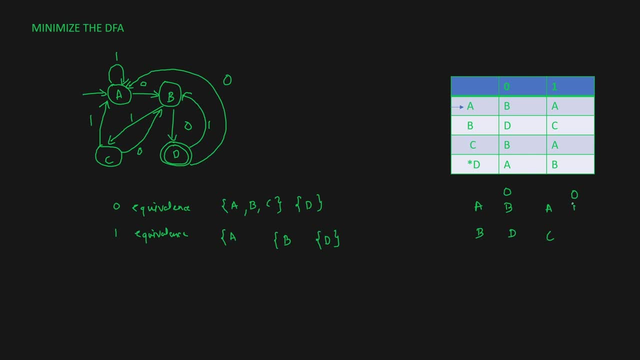 On getting input zero, A is going to B, Okay, And what about C? C is also going to B, Fine. Now what about input one? So, on getting input one, A is going to state A, Okay. So we are comparing this. 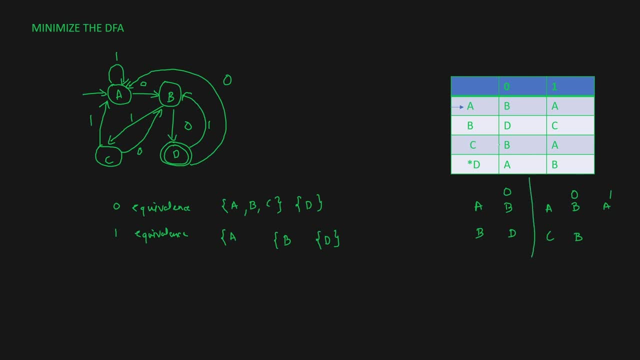 Okay, We are comparing A and C, Yeah, And on getting input, one C is also going to state A. Okay, So that's why A and C are one equivalent. So A comma, C. Alright, Now we have got three groups over here. 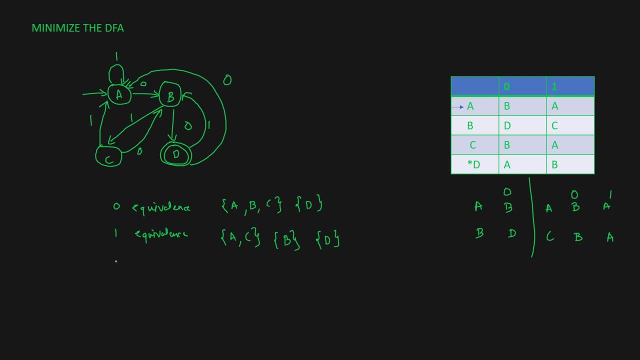 A comma, C, B and D. Fine, Now you have to check for two equivalents. Same processor, Okay, Two equivalents, Alright. So now you compare A and C. Since we already know that A and C, on getting both input zero and one they are getting, they are going to state B and A. So that's why A and C are. 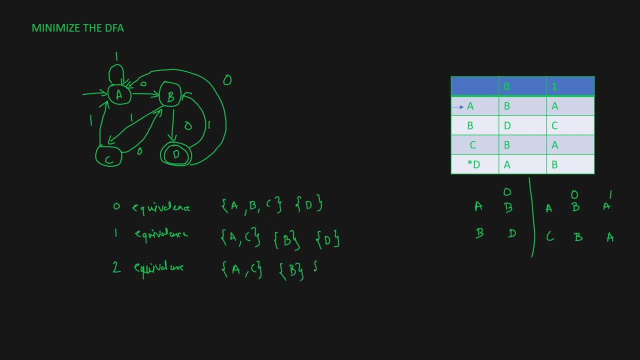 two equivalent Alright And B. there is nothing to compare, and neither there is anything to compare with D. So once you get two back to back equivalent states, you conclude and you stop there. only So we have minimized this DFA. Now let's construct and combine these two states. 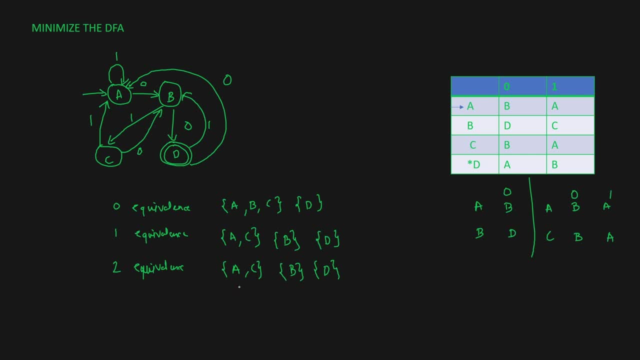 That is, A, comma, C combined into one single state and construct our new DFA. Okay, So how does the transition table will look like? So let's draw the transition table over here. Okay, So let's say we have got our three states over here. 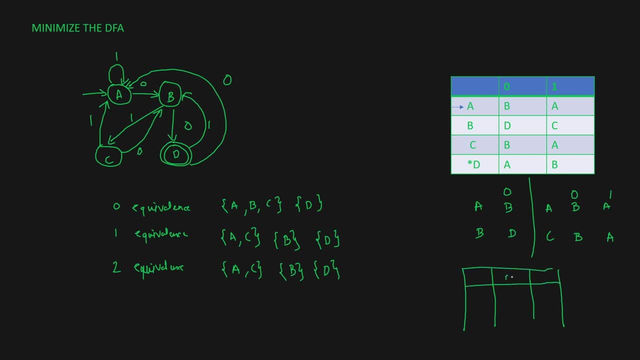 Okay, First let's write the input zero and one- And This is our first state- combined state A, C. Okay, So, on getting input zero, A, C is going to state B, And on getting input one, it is going. 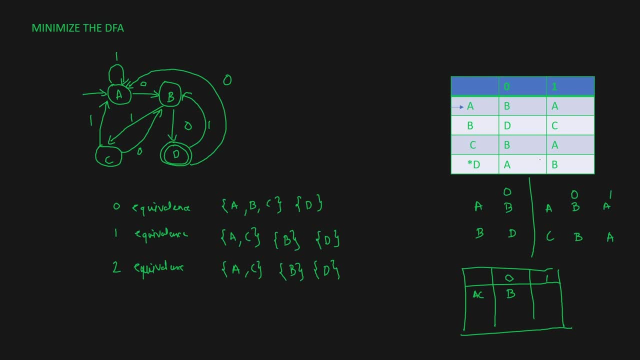 to state A, But there is no state A. We have got a new state. It is known as A, C, Correct, Fine. What about the next one? That is B? So on getting input zero, it is going to state D, And on getting input one, 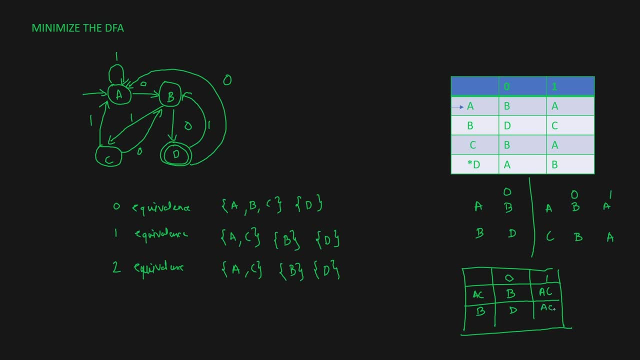 it is going to state C, But there is no state such as B. Okay, There is no state such as C. It is A- C. Okay, Now we have got our final state, That is, state D. Final state On getting input zero: it is going to state A, But we have created a combined state called. 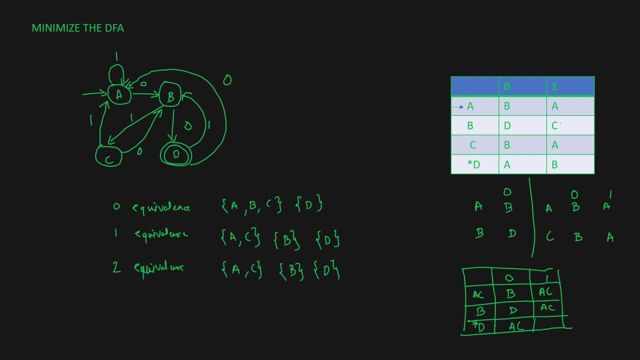 as A C. So it is going to state A- C And on getting input one, it is going to state B. Alright, So this is our starting state A C, then state B and final state is D. Now let's draw this. 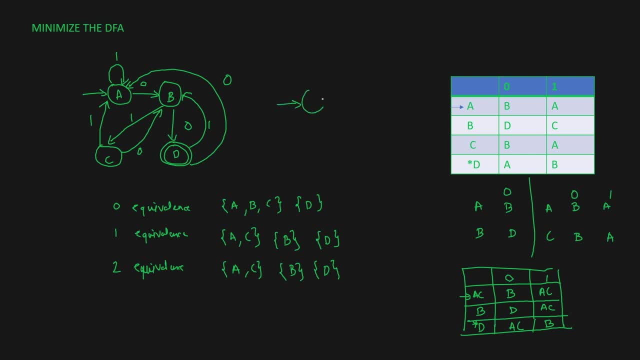 DFA and see how it looks like. Okay, So this is our starting state. On getting input 0, it is going to state B. On getting input 1, it is staying in state AC. What about state B? On getting input 0, it is going to state D. And on getting input 1, it is going to state. 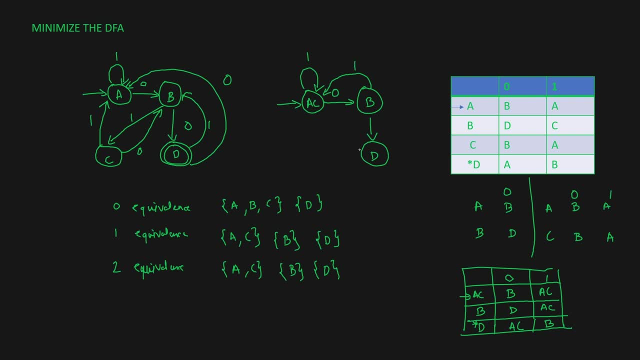 AC. And what about state D? It is a final state. On getting input 0, it is going to state AC And on getting input 1, it is going to state B. So this is how we have minimized the DFA from 4 states to 3 states. 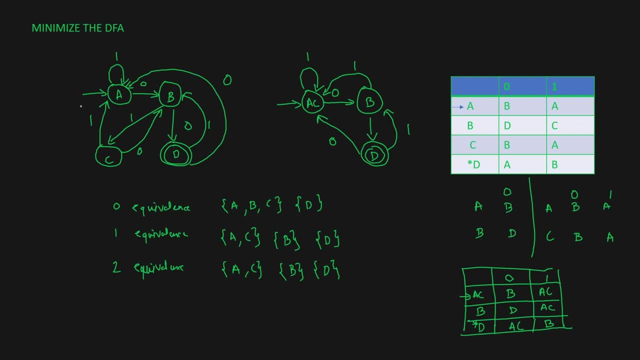 Now let's try to pass a string and see if it works out or not. So let's say we pass a string like 0010.. Let's try this string: 0010.. 0010, 0010, 0010, 0010. 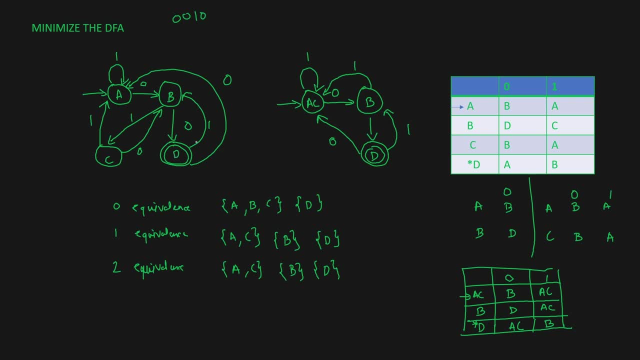 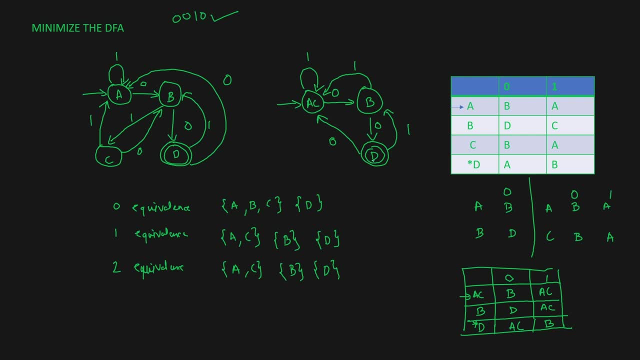 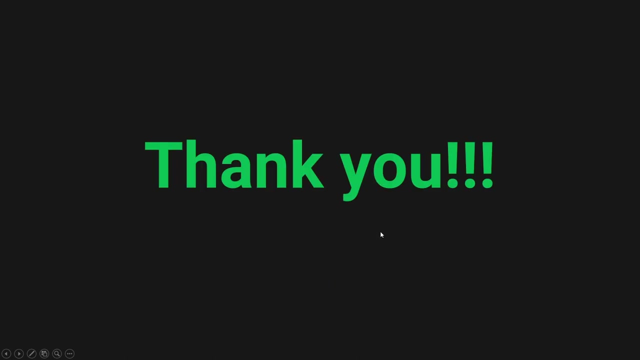